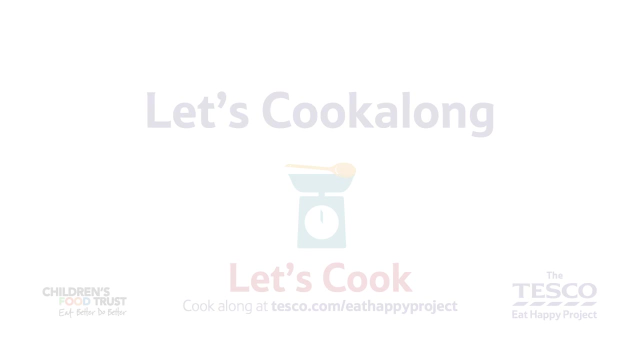 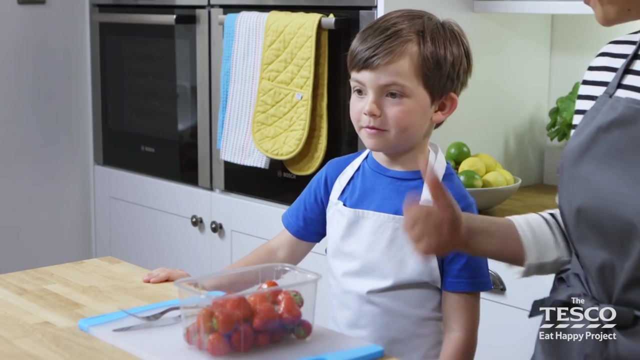 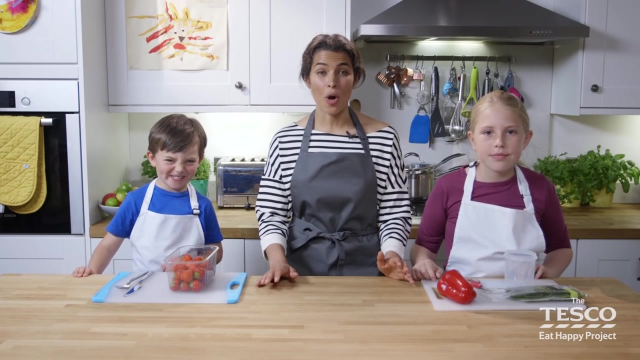 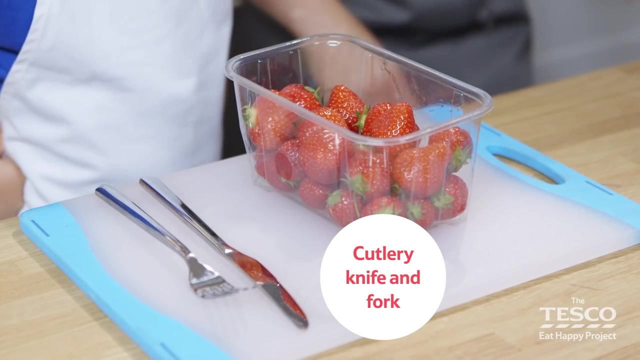 Hi. this is Liberty, Hello, And this is Milo, Hello. Have you washed your hands, guys? Are you ready to go? Brilliant, We're going to teach you different ways to chop. You'll need a chopping board, scissors, a sharp knife, a beaker and a cutlery knife and fork The. 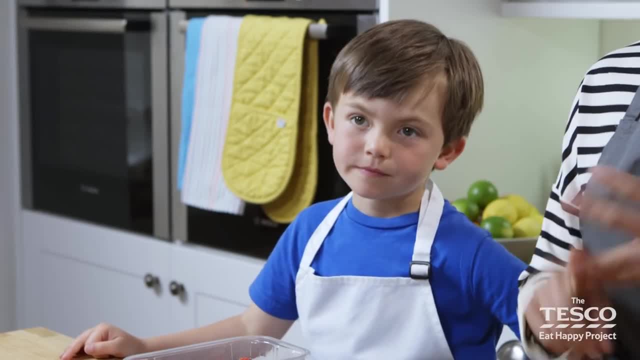 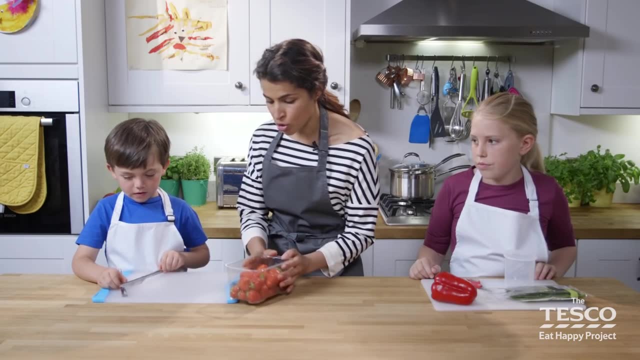 reasons we chop things is to make them smaller. This is because we can cook it more quickly and it's easy to eat, and sometimes it makes it look a bit nicer as well. What we're going to do today, Milo, is get you to chop some strawberries. This is a really good technique for smaller. 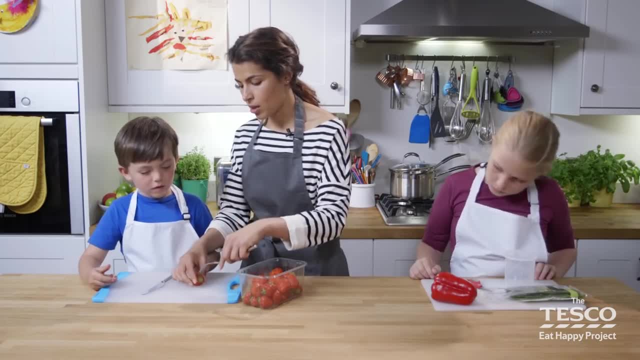 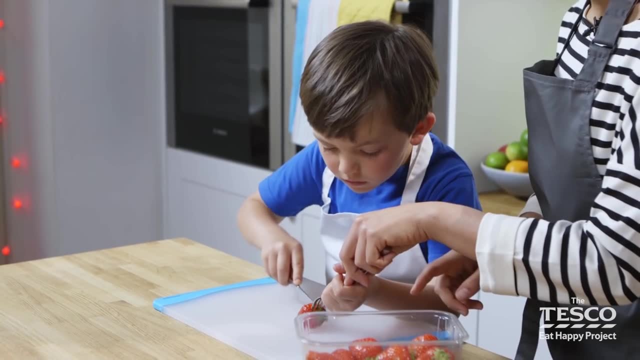 children to allow them to have some stability when they're cutting. You hold the fork through the actual fruit. This is called a fork secure technique. So we're going to use a cutlery knife to cut through this strawberry with Milo. We've used the fork and its prongs as 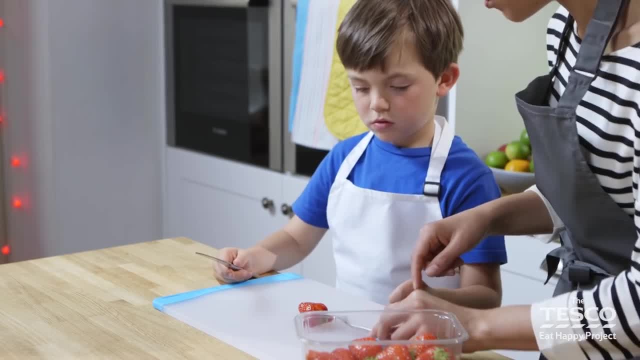 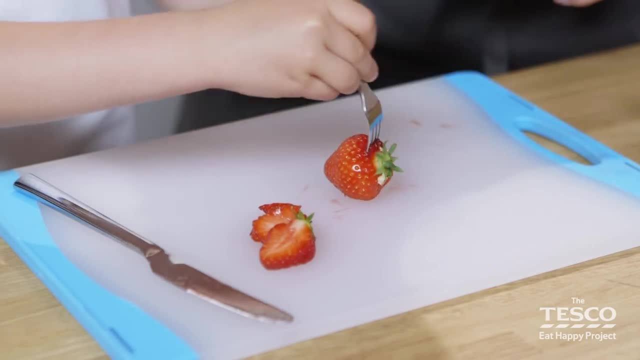 a really good guide to help cut through and slice them into even pieces. Well done, Milo. you did that really well. Can I get you to do another one? I'm going to leave you to do this one, so you know how to stab it. Stab ya, That's a good boy. I think you're a pro. 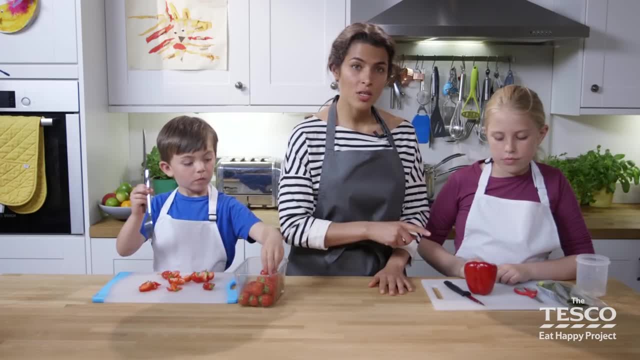 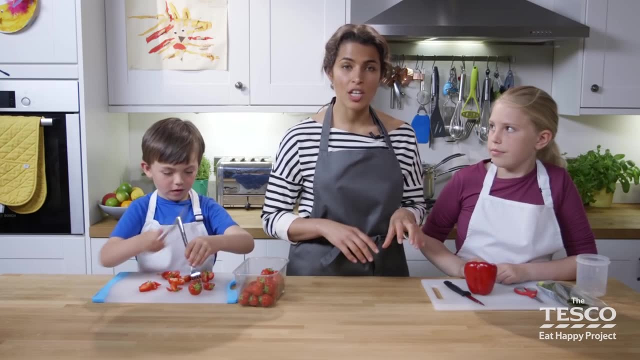 Well done, Milo. So whilst Milo's chopping through the strawberries, I'm going to show you with liberty how to chop a pepper. There's really two very important techniques when you're chopping. There's a hold called the bridge and another one called the claw. These 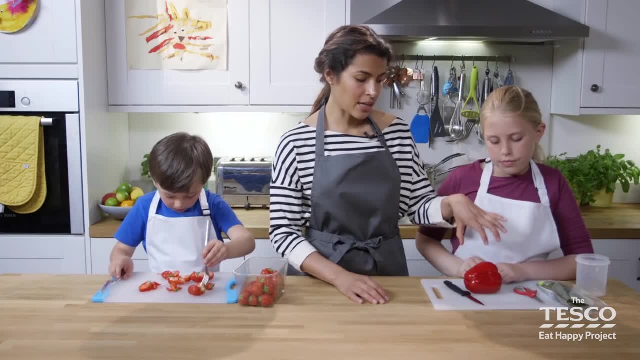 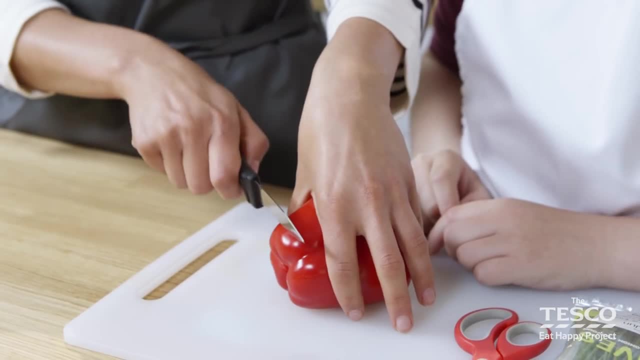 are really good ways of cutting safely. We're going to have to use the bridge technique, which is basically using a tunnel shape over the top of the pepper like this, with your thumb behind, to take off the bottom. If an item of food's not even in shape, it's better. 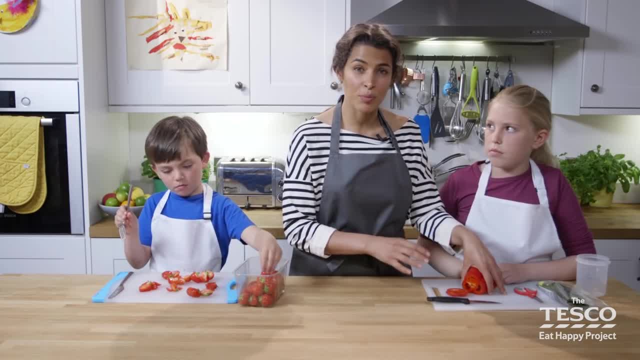 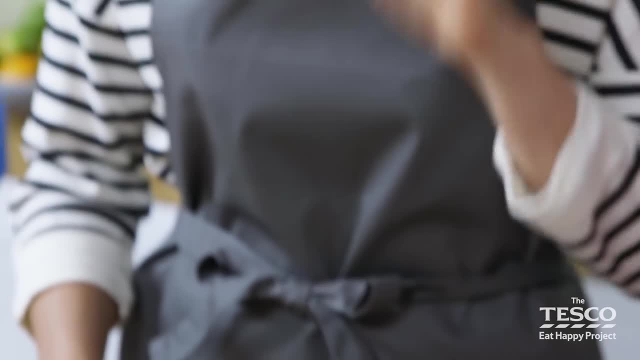 to chop off the bottom. We don't want it rocking and rolling on the surface of the chopping board. Obviously, accidents could happen And turn it over, and then I'm going to get Liberty to show you how to use the claw. You need to make a claw like this, Then put it on the. 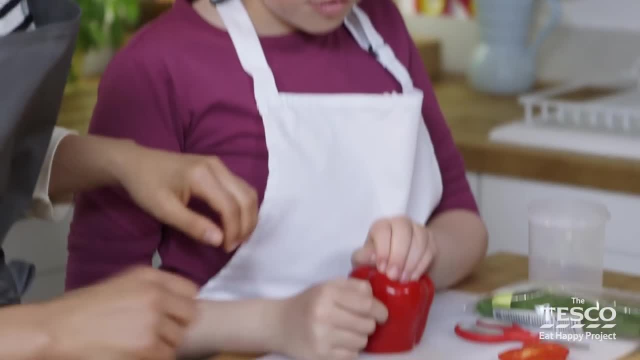 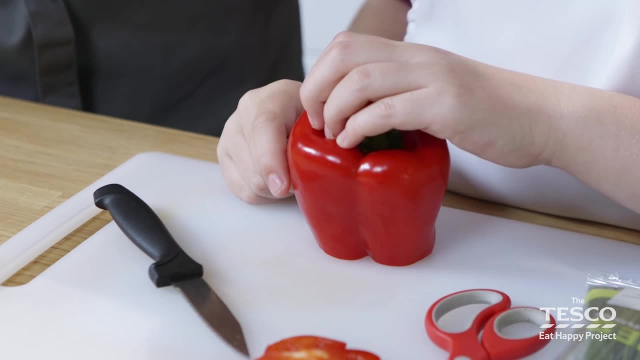 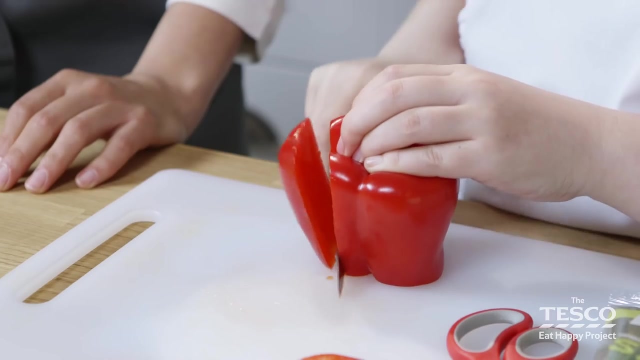 food when you're going to chop it like this. Well done, Liberty. fantastic. Keep your fingers close together. It's a bit like a bear claw: It keeps your fingers away from the knife, but lets you actually hold the item in place. That's it. Oh wow, you're a professional in this, Liberty. Have you done it before, Can?